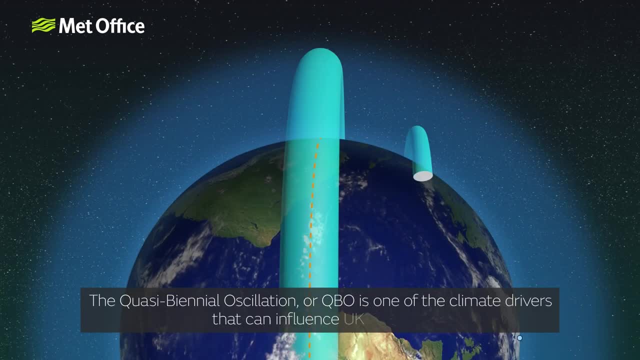 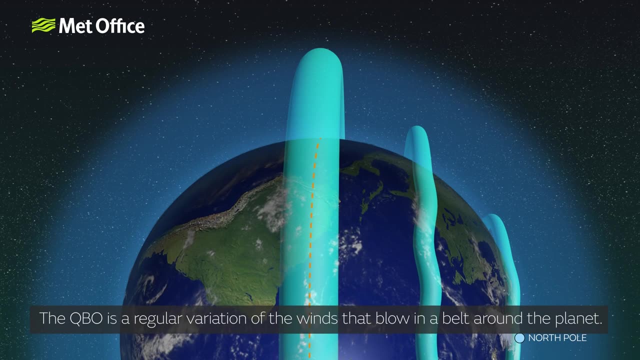 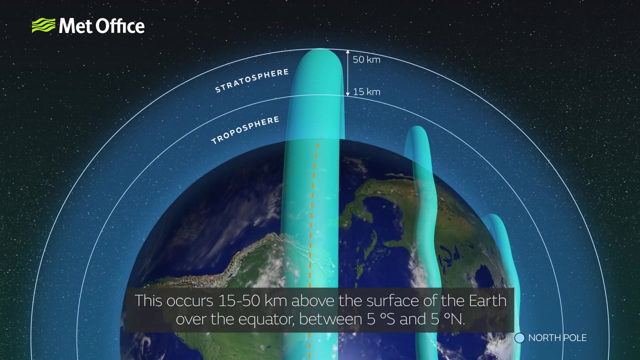 The Quasi-Biannual Oscillation, or QBO, is one of the climate drivers that can influence UK weather. The QBO is a regular variation of the winds that blow in a belt around the planet. This occurs 15 to 50 kilometres above the surface of the Earth, over the equator. 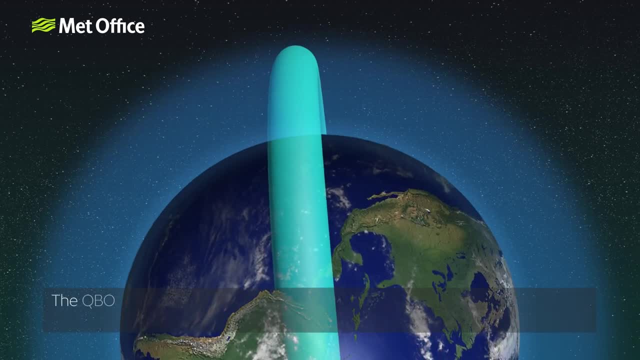 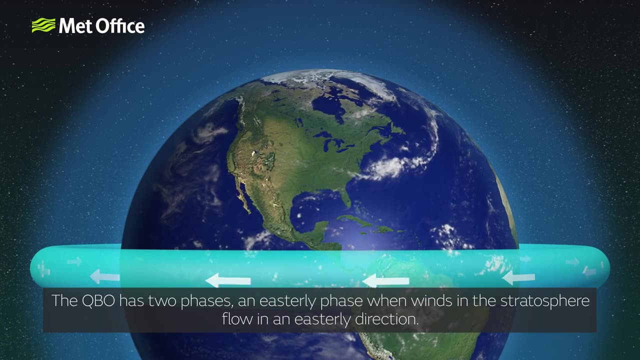 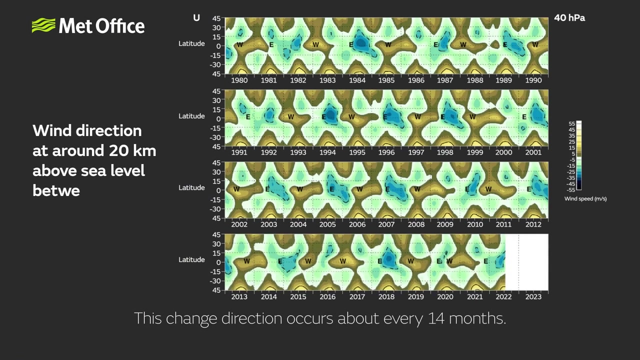 between 5 degrees south and 5 degrees north. The QBO has two phases: an easterly phase, when winds in the stratosphere flow in an easterly direction, and a westerly phase when the winds change to a westerly direction. This change in direction occurs about every. 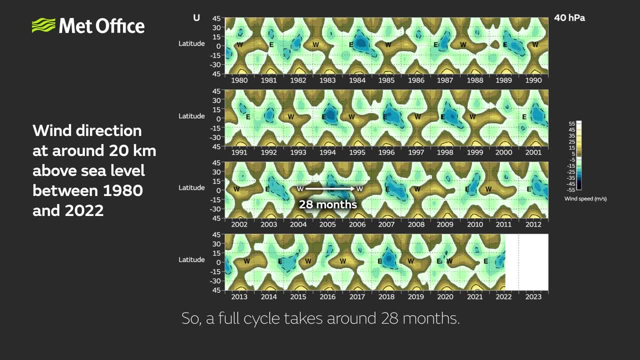 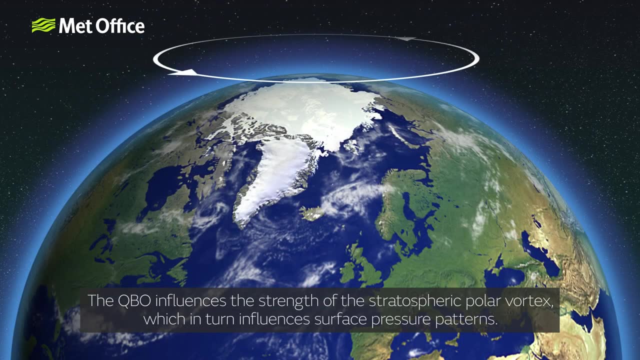 14 months, so a full cycle takes around 28 months. The QBO is one of the most regular atmospheric oscillations, making it highly predictable. It has wide-reaching impacts and can affect UK weather. The QBO influences the strength of the stratospheric polar. 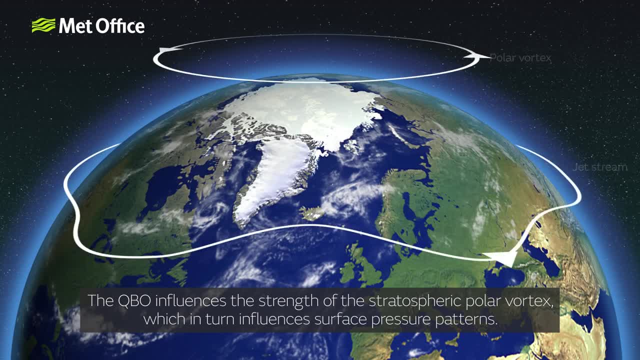 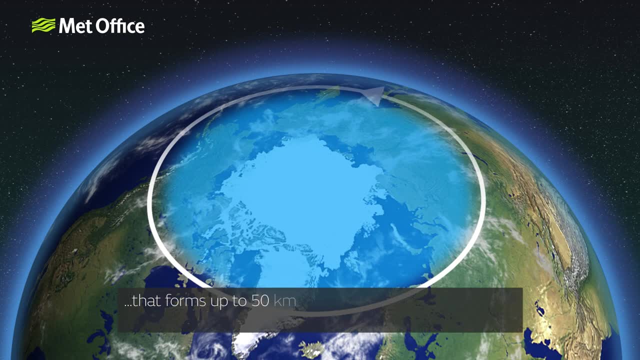 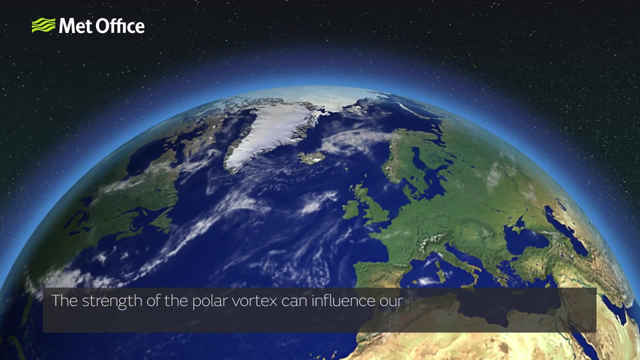 vacuum. The stratospheric polar vortex is a fast-moving circulation of stratospheric air that forms up to 50 kilometres above the surface of the Earth around the North Pole. in winter, The strength of the polar vortex can influence our jet stream, which is a core of strong 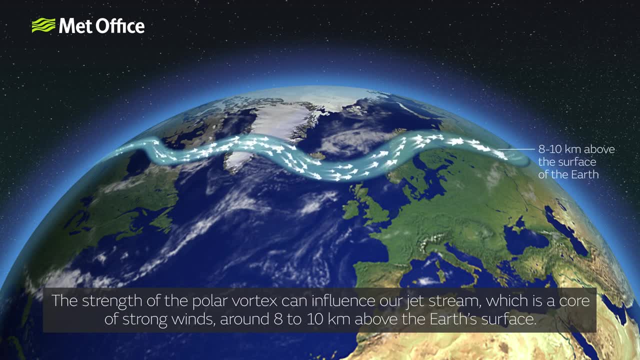 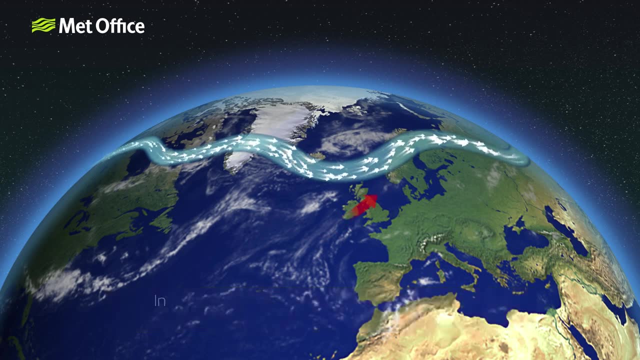 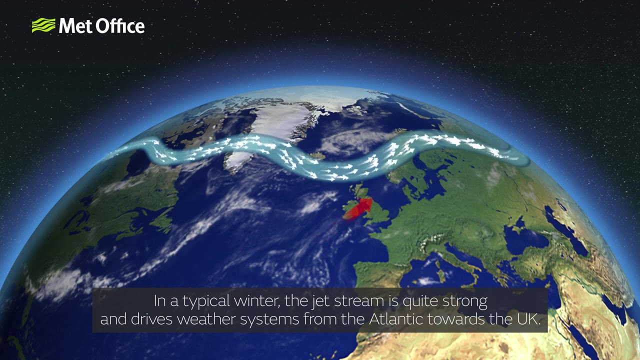 winds around 8 to 10 kilometres above the Earth's surface. We normally expect UK weather to come in from the west with a flow of relatively mild air off the Atlantic. In a typical winter the jet stream is quite strong and drives weather systems from the Atlantic towards the UK When the QBO is in a westerly phase. 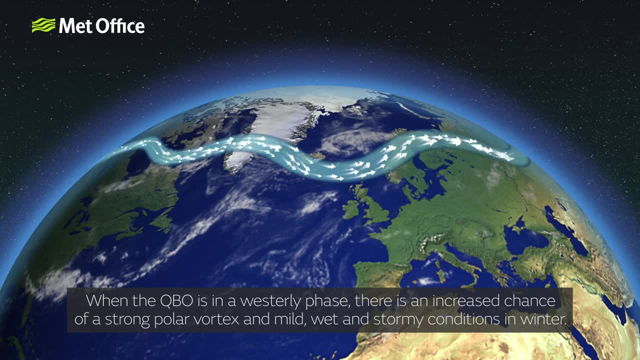 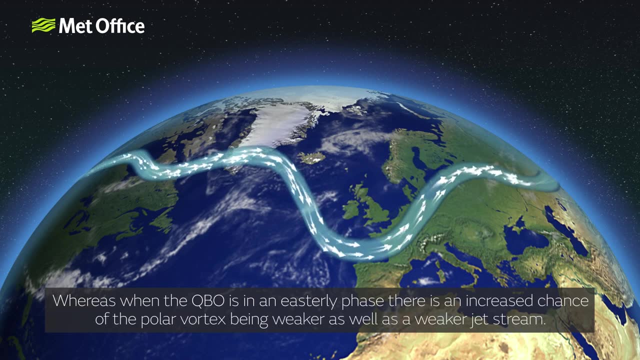 there is an increased chance of a strong polar vortex and mild, wet and stormy conditions in winter, Whereas when the QBO is in an easterly phase, there's an increased chance of the polar vortex being weaker, as well as a weaker jet stream. 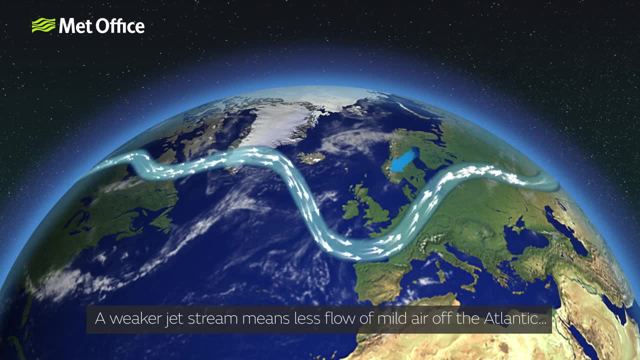 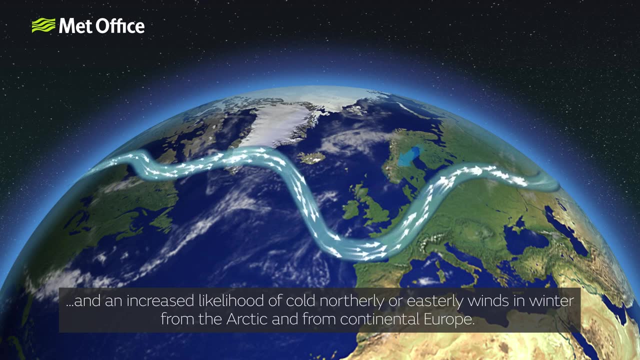 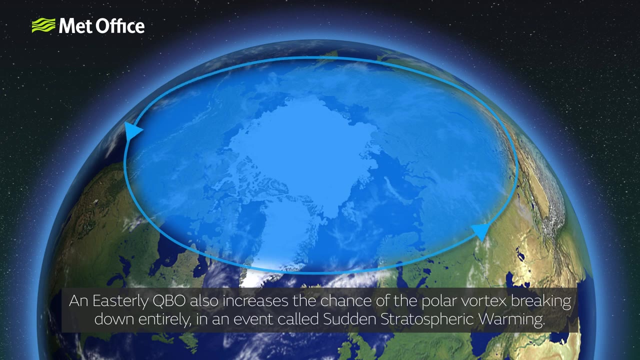 A weaker jet stream means less flow of mild air off the Atlantic and an increased likelihood of cold northerly or easterly winds in winter from the Arctic and from continental Europe. An easterly QBO also increases the chance of the polar vortex breaking down entirely.